can't see the ones below that because the Earth is in the way, But if you're lucky enough to live near the equator, you can see all the constellations over the course of a year, Which brings us to another point. The constellations that you can see don't just depend on where. 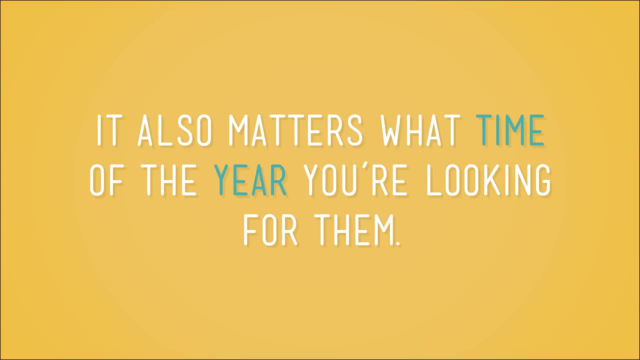 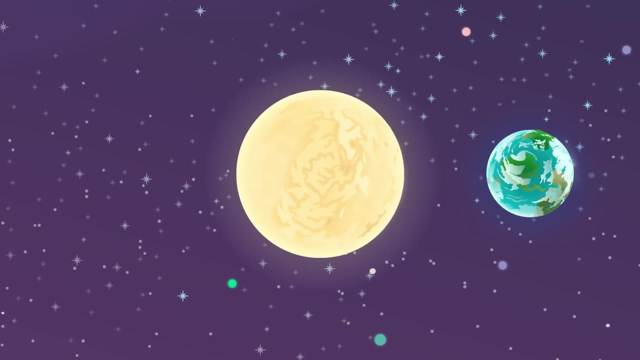 in the world you are. It also matters what time of year you're looking for them. To see why this is, let's take a look at Ursa Major. Hey, there home planet. Here's the Sun over here and all those twinkly things are stars. 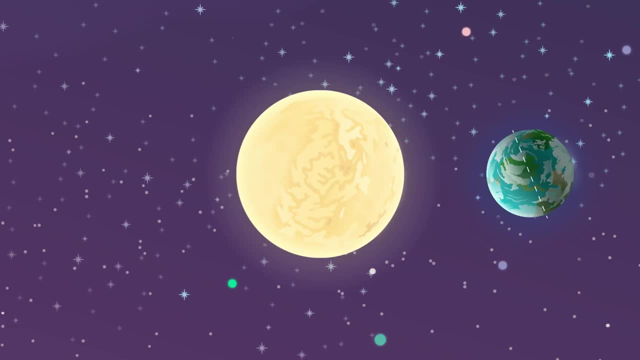 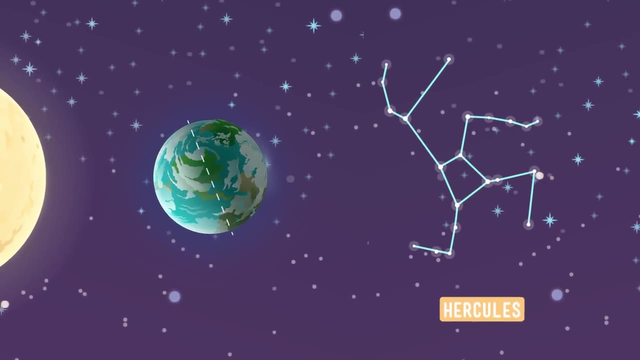 and constellations. You'll notice the right side of the Earth is darker than the left side. That's because it's nighttime on that side of the Earth, So people on this side of the planet have a great view of the stars and constellations over here As the Earth. 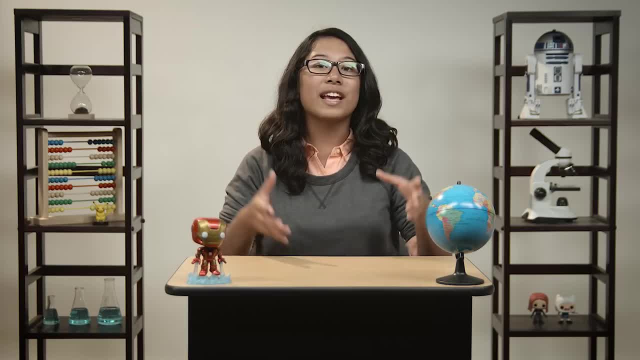 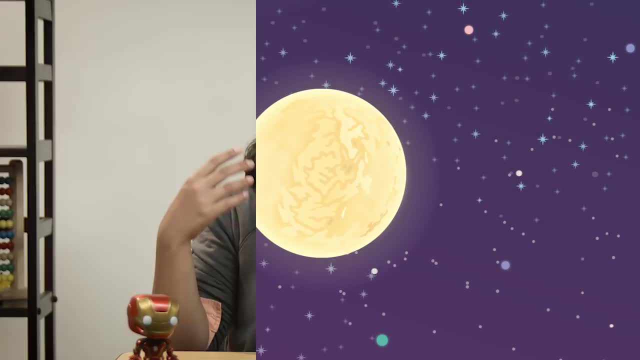 rotates on its axis. whichever part of the planet is facing away from the Sun has a great view of these stars. during this season, Let's say, it's winter if you're in the northern hemisphere and summer if you're in the southern hemisphere. But, as you know, the Earth isn't. 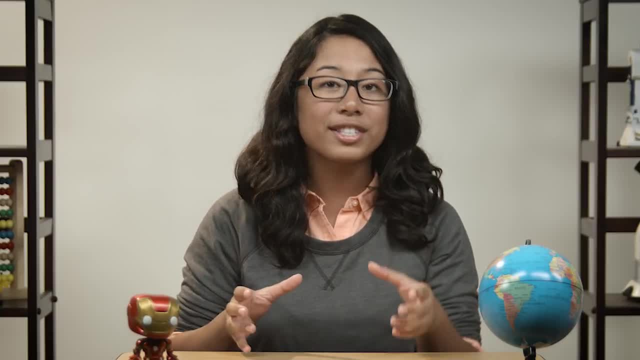 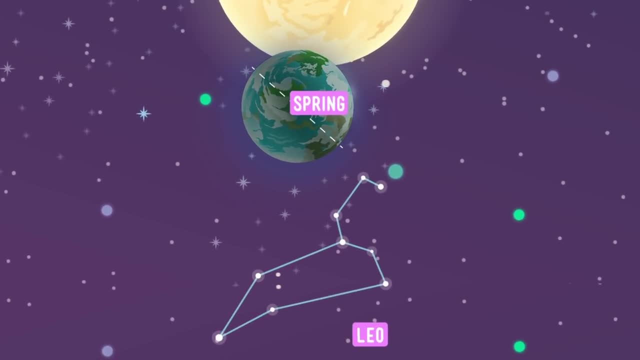 just spinning on its axis, It's also revolving around the Sun. So as the Earth moves around the Sun, the seasons change From, say, winter to spring Or, in the southern hemisphere, summer to fall. And as the seasons change, so do the constellations that are visible. 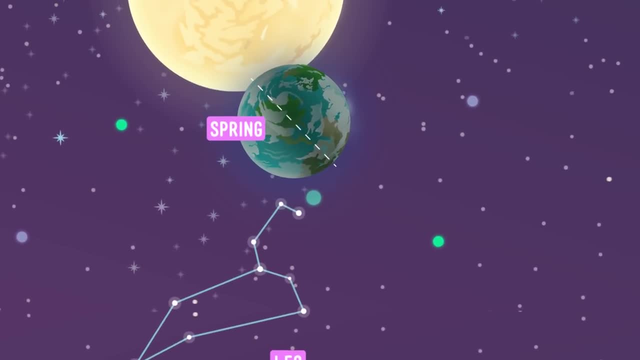 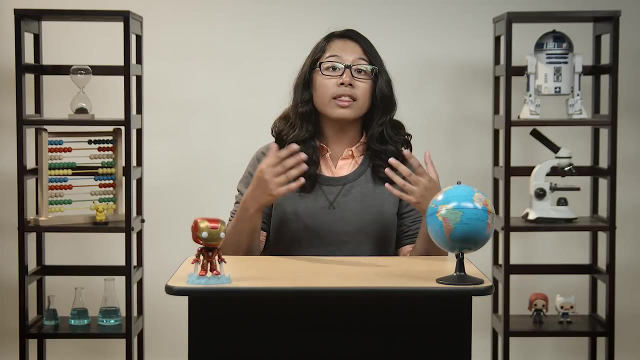 at night. So several months later, you're now seeing these stars in this part of space, And as the Earth continues around the Sun, the seasons change from spring to summer or fall to winter in the south, And these stars are now visible to us at night. 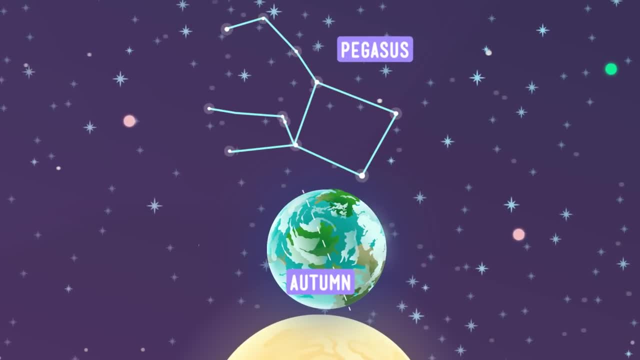 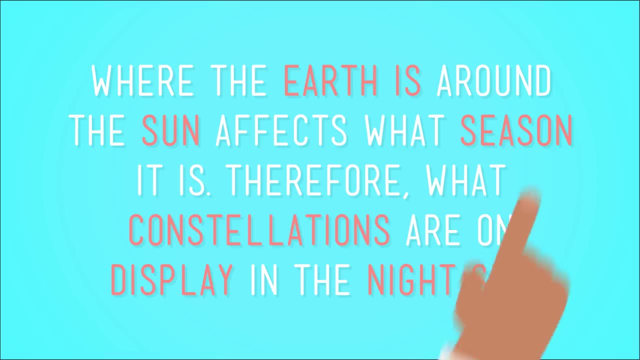 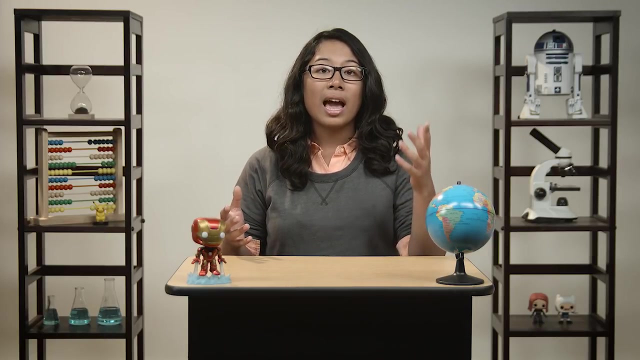 And as the Earth continues its path around the Sun, giving us this group of stars. So where the Earth is around the Sun affects what season it is and therefore what constellations are on display in the night sky. And that helps us tackle our big question: How do the constellations appear to move across? 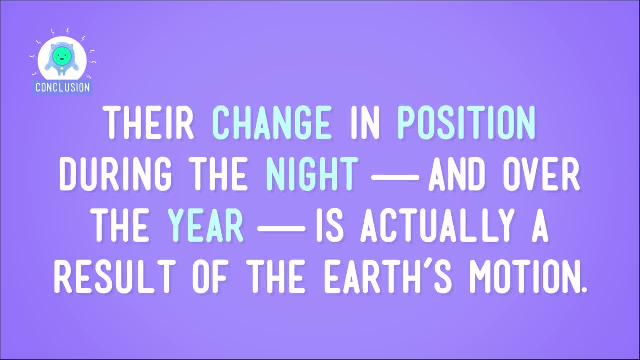 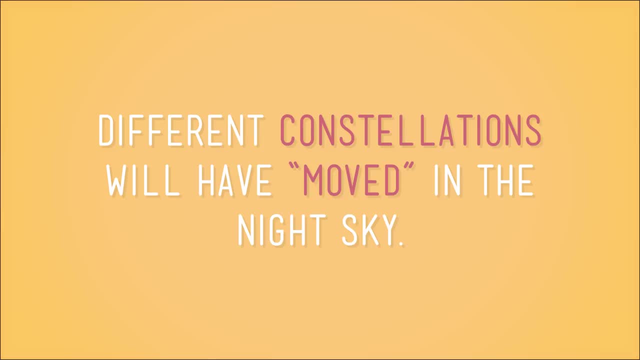 the night sky. Their change in position during the night and over the year is actually a result of the Earth's motion. Depending on where in the world you are and when you're looking, constellations will have moved into view in the night sky. 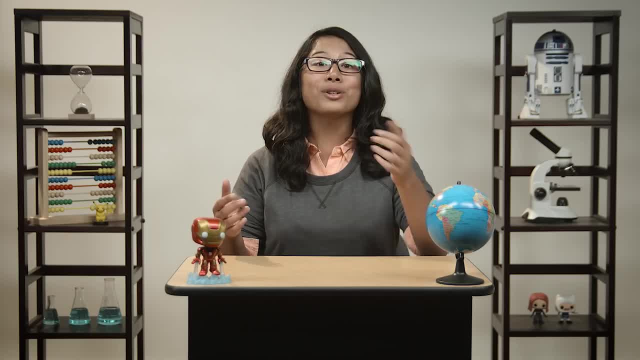 What constellations are visible where you live this time of year. To find out, just grab a few friends, maybe some nice hot chocolate, and wait for dark to do some serious stargazing. 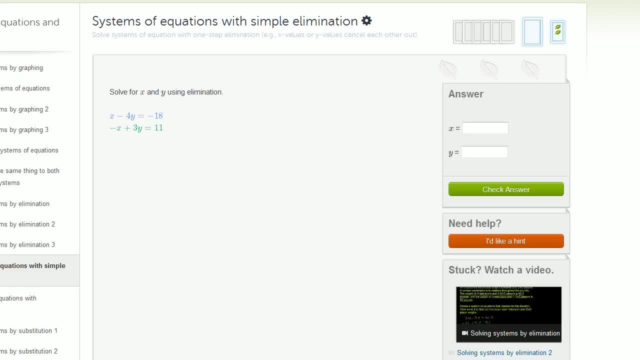 Just in case we need to help with more party planning for the king, let's get ourselves some practice with solving systems of equations with simple elimination. And so here's the exercise right over here We have: x minus 4y is equal to negative 18.. And negative x.